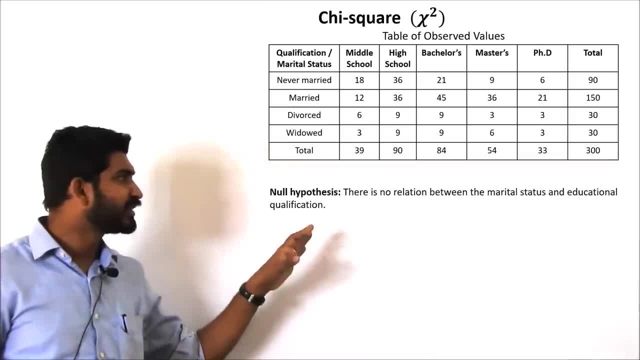 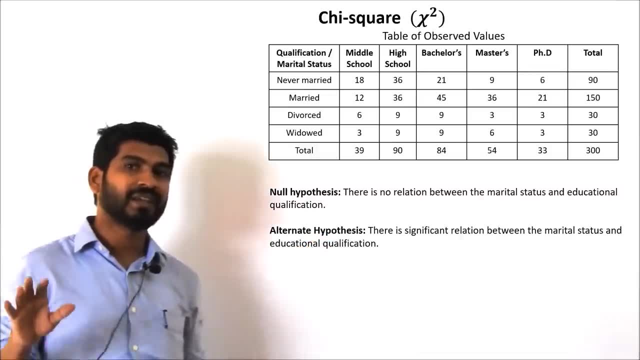 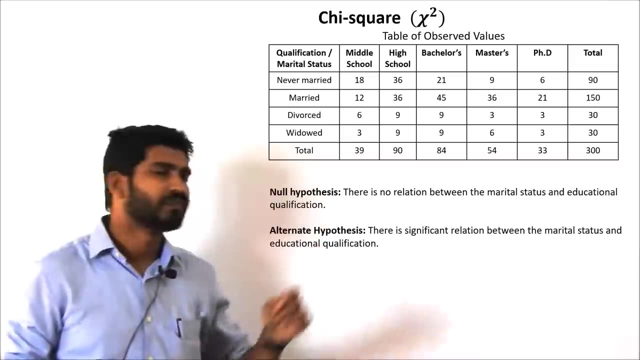 and the alternate hypothesis. Our null hypothesis can be stated that there is no correlation between the two variables, and the alternate hypothesis can be stated by saying that there is significant relation between the two variables. Now, significant, the significance level is to be defined, The significant level: either it can be taken as 0.0 or 0.0.. So 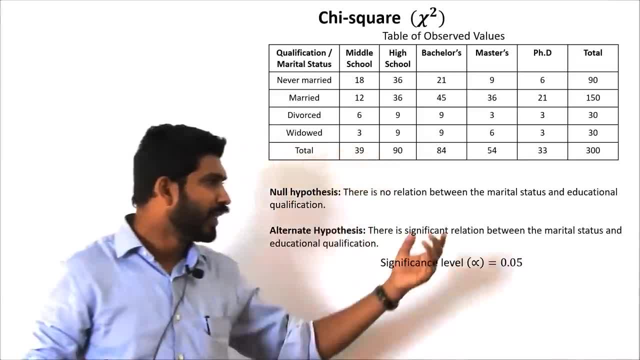 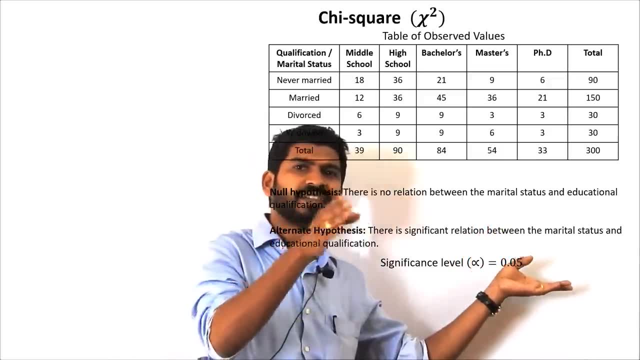 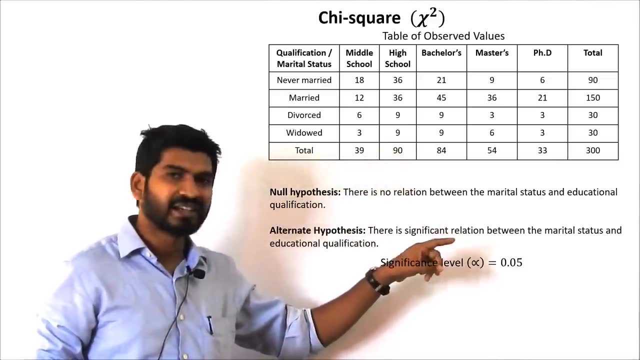 0.05, which is 5% deviation from the mean, or we can say 0.01.. Usually the significance level is taken as 0.05.. There are different significance levels taken for different type of observations, But generally the significance level is taken as 5%, that is, 0.05.. So we 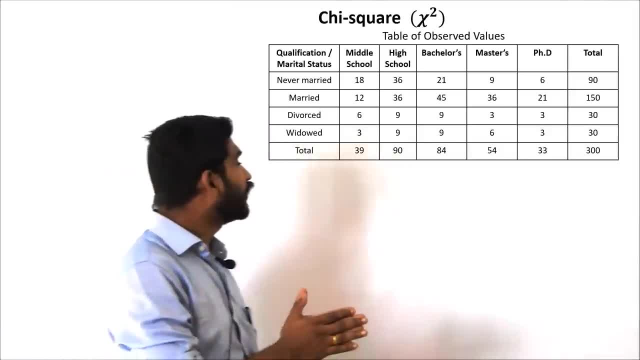 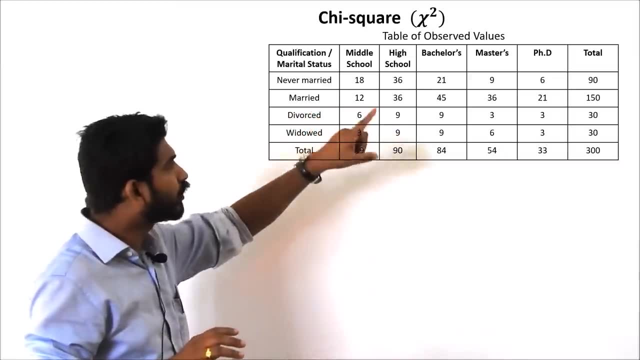 will go with that Now. how to start Now? first of all, we will look at the observation values, the values which are observed or which have been taken from the field, So these are called as observed values. Now we will prepare another table for the. 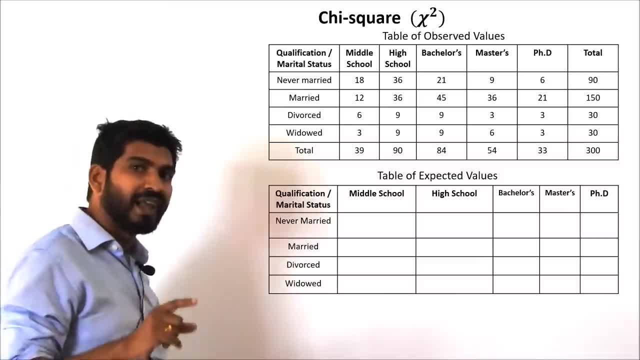 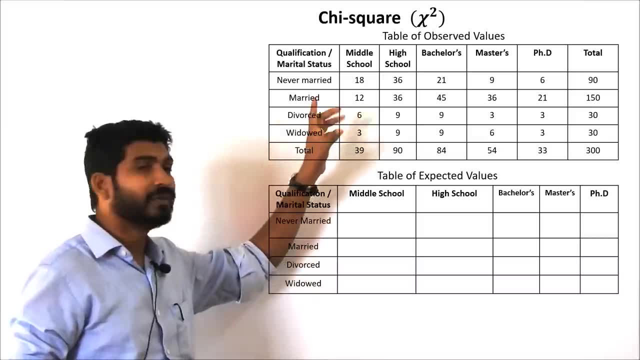 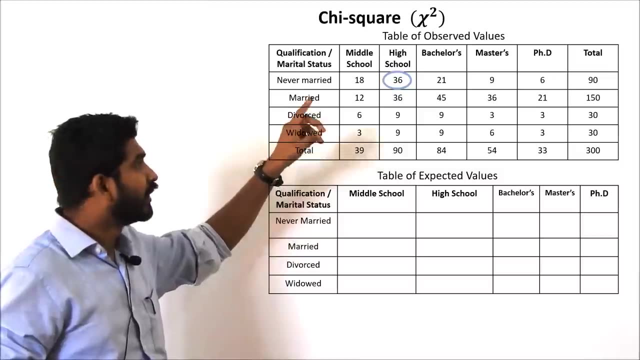 same variables, but those values will be calculated values, or you can say the expected values. Now, how to calculate it? Now, in this table we can see there are 36 people who are unmarried and whose education is high school. right Now, for those people, the expected value: 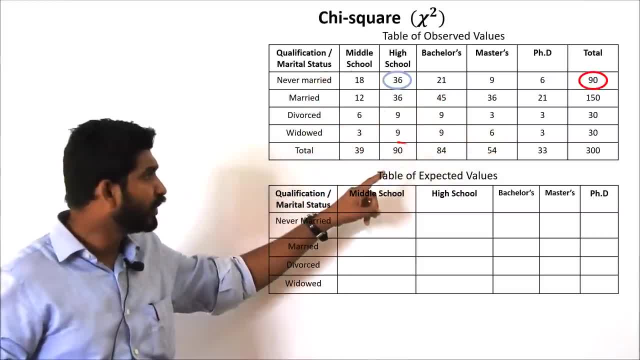 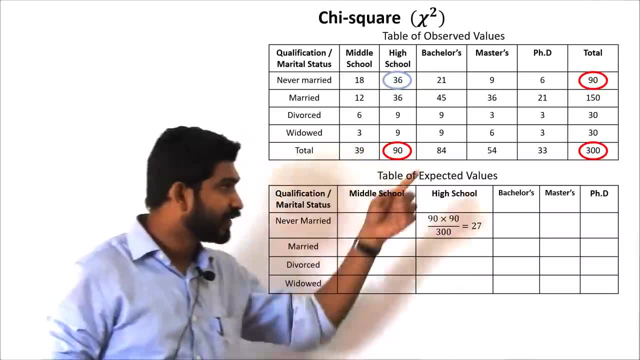 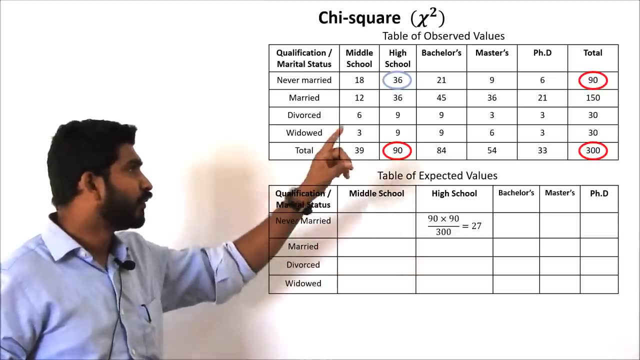 could be The row total into the column total divided by the grand total. There are 300 people whose data has been collected, So that is called as the grand total, So that comes out to be 27.. In the same way for the first element, that is 18.. There are 18 people who 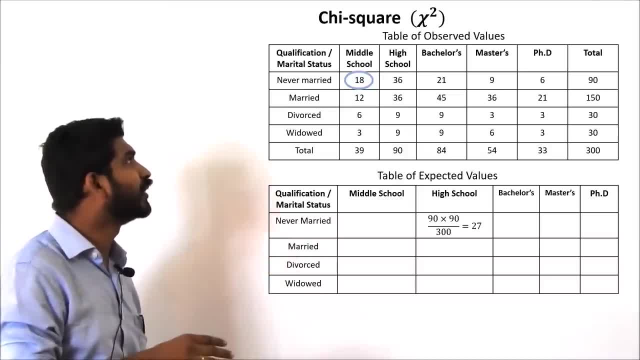 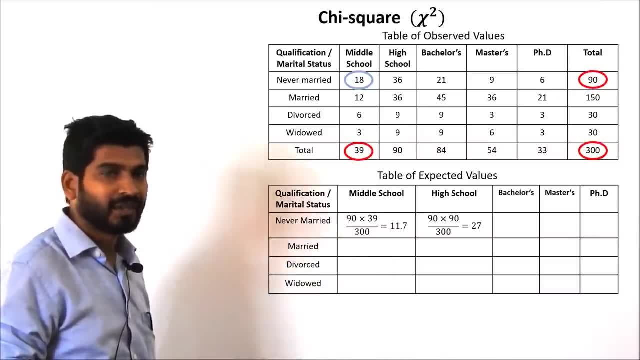 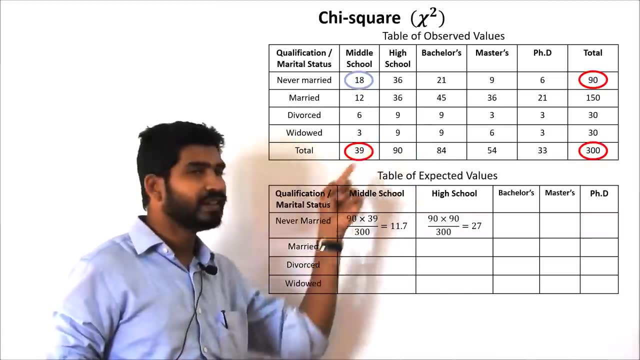 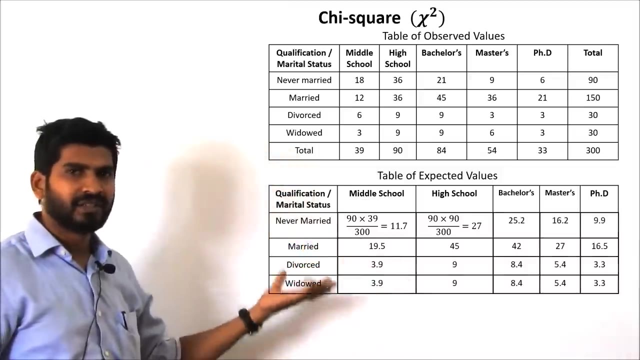 are unmarried and whose education is middle school. The expected value will be 90 into 30.. 39 divided by 300. That will give you 11.7.. In the same way, we need to calculate the expected value for all the categories and the table, which will get like this: This will: 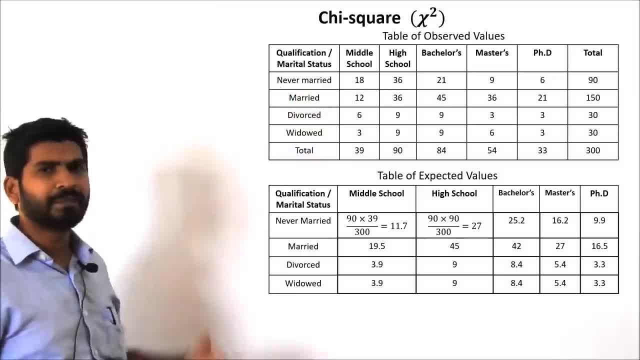 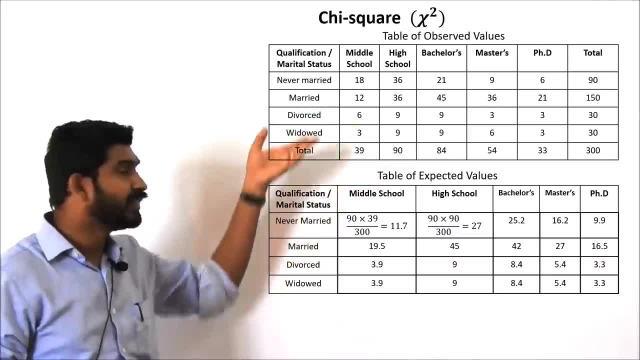 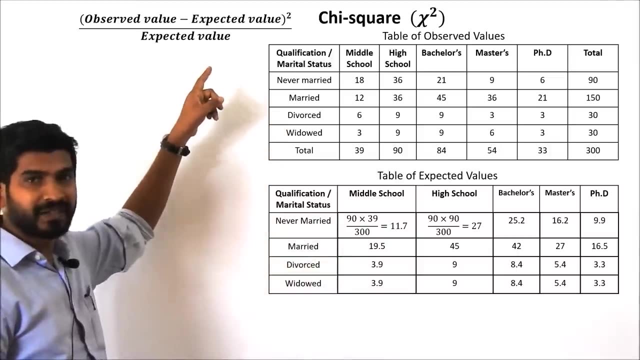 be the table for the expected values, and the first one was the table for the observed values. Now our aim is to find out how much deviation is there between the two given values. That is founded by a simple formula that is observed minus the expected value, the whole. 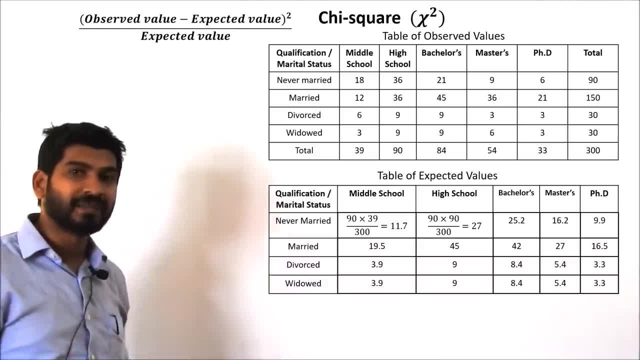 square upon the expected value. So we prepare another table which states the difference between the two variables, which states the difference between the two values. okay, Now we will look at this table now. Here you can see the table contains different values. 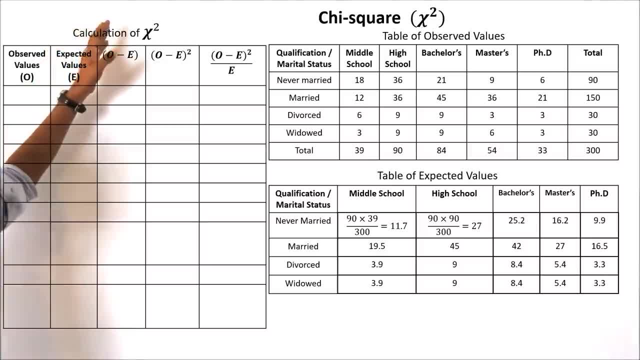 The table contains the observed value, the expected value, the difference between the two values, The square of the difference between the two values and divided by the expected value. So we will fill out this table. The first value there was 18, and the observed value. 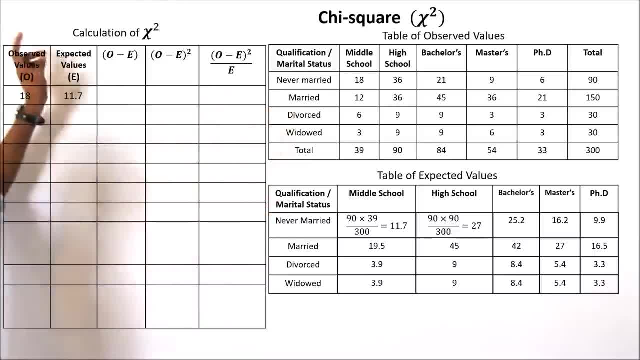 was 18.. The expected value is 11.7.. So 18, 11.7, the difference, the square, and we divide it by the expected value, that is 11.7.. What I get is 39.69.. And once I divide it by the 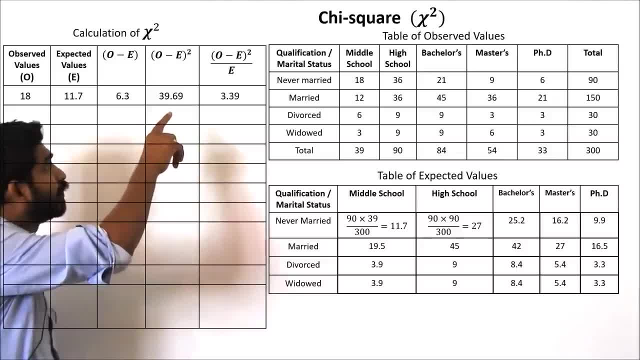 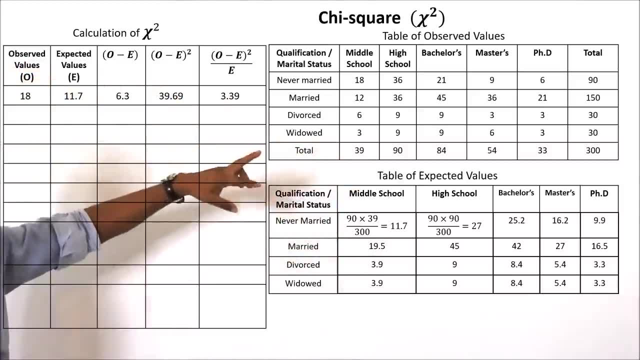 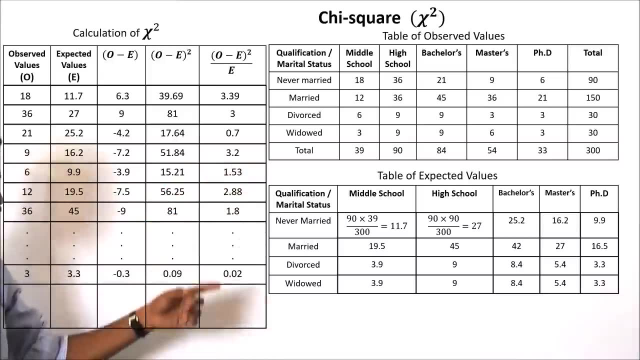 expected value, I get it as 3.39.. Now, in the same way, we need to calculate all the given values, the difference between the expected and the observed values, and I get this table completed. And once I complete this table, you can see the total of this last column. 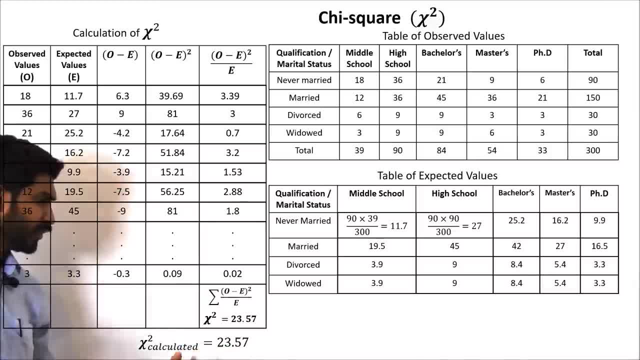 that is the observed value minus the expected value, the whole square upon the expected value. So this is the value of the chi square. Now, this value is the calculated chi square. We also need to compare this value with the tabular value of chi square. Now, how is that? 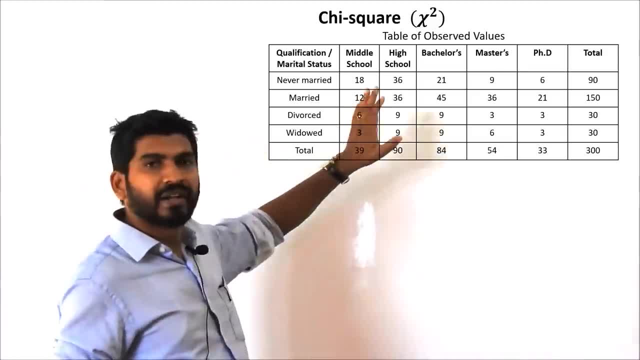 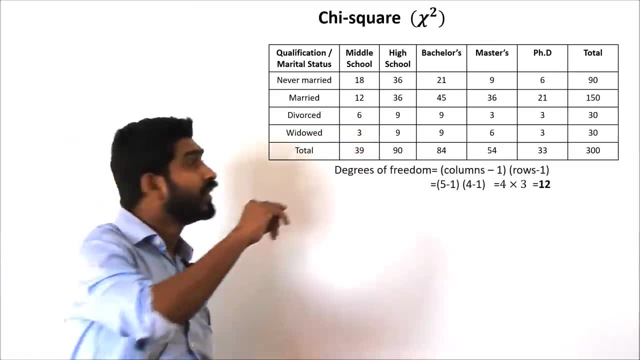 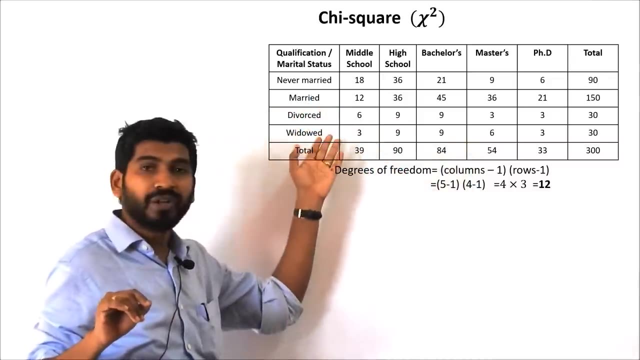 calculated. Now for tabular value, I need to find out the degrees of freedom. Now, degrees of freedom is found out by a simple way. You can see in the original question there were 5 columns, 5 different categories for the level of education And there were 4 different. 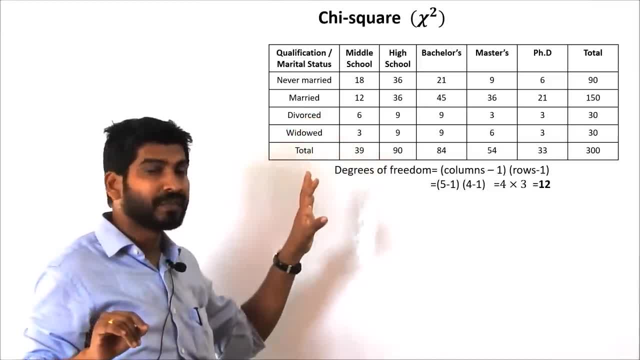 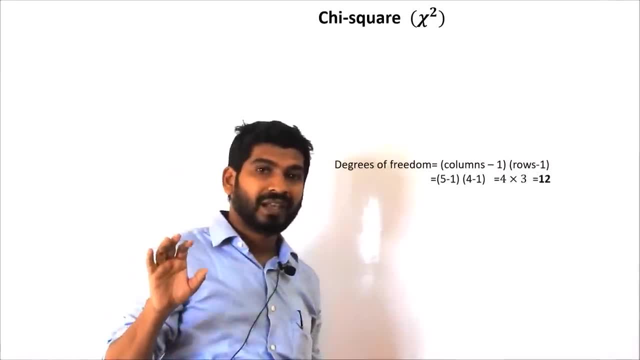 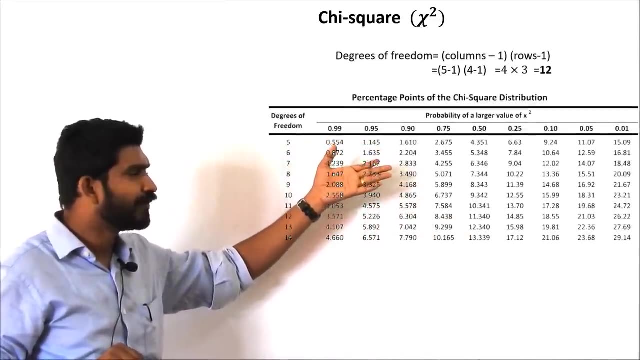 degrees for the marital status. So the degrees of freedom is calculated by 5 minus 1 into 4 minus 1, that comes out to be 12.. So 12. we need to see the table for the. we need to see this table for the tabular value of chi square and we can see the tabular value.